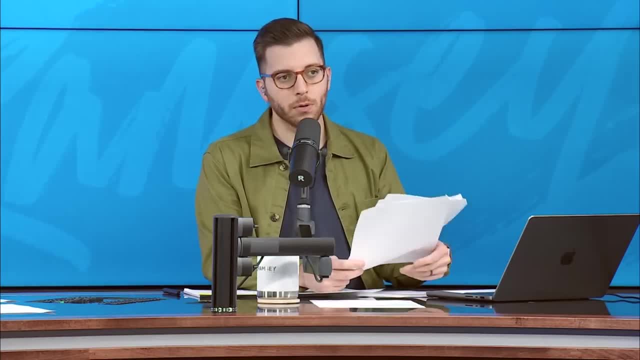 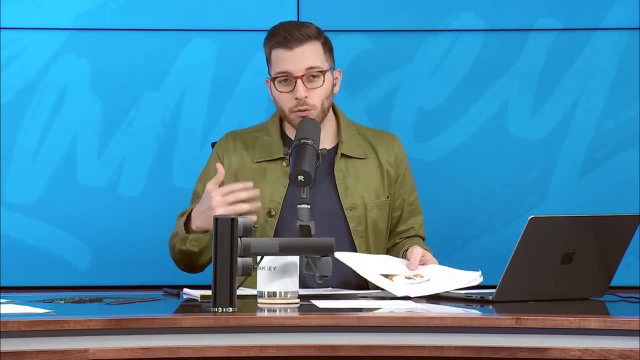 let's talk through an example of this and the power of starting early, Because a lot of people- they aren't- maybe they're not there yet, Ken- Either they have debt, they don't have the emergency fund, They're in their 40s or 50s or 60s- They feel like it's too late. They feel 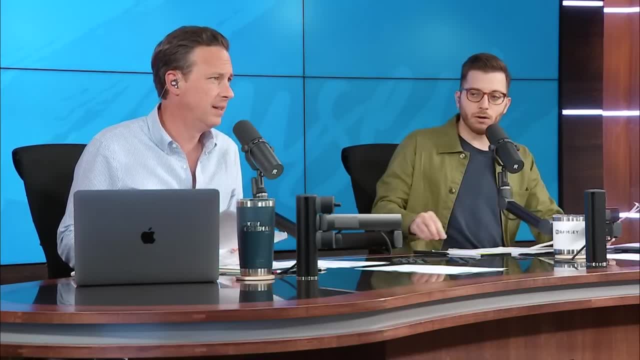 like they don't have the knowledge base. I like that. Let's take someone my age, George, I'm 48. Oh boy, All right, I wasn't going to go, that old Ken, I was going to go. 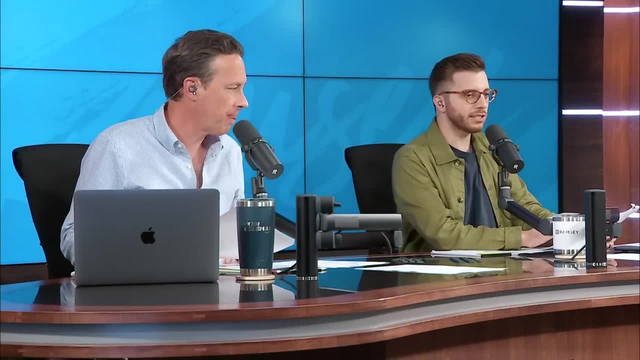 Well, the example here. you can change the numbers on the example, But let's say this guy, Ben, who starts at 21. 21. He's a kid, His parents went through FPU, He did this stuff And he invests $2,400. 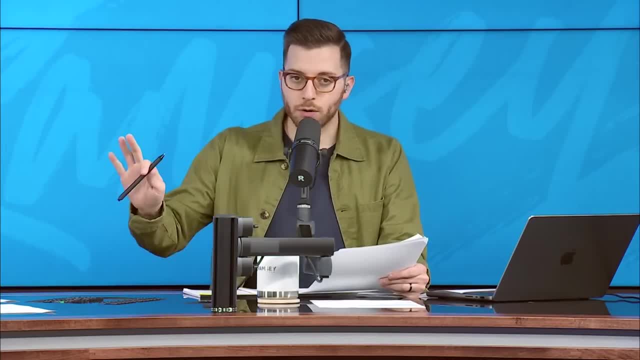 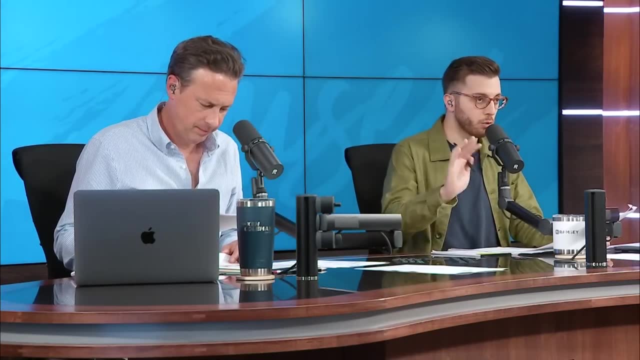 a year. You got that Just $2,400?. $2,400 a year, That's not a lot. That's $200 a month, Yeah, And he stops contributing at age 30. So from 21 to 30, $2,400 a year The total amount. 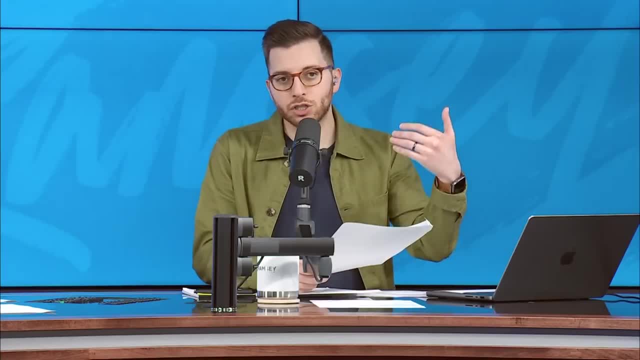 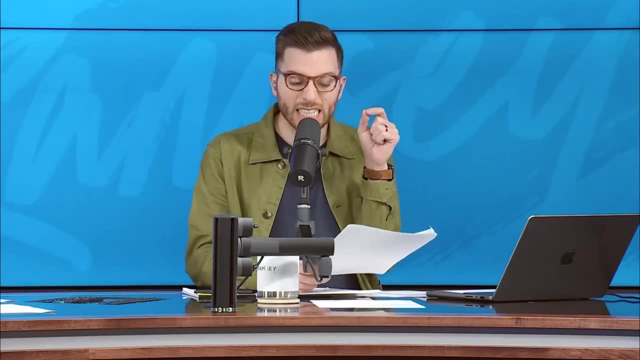 he contributed was $21,600.. Now his buddy Joey, a little older, he started investing at age 30. And he invests $2,400 a year as well, And he contributes until he is 67. So instead of nine years he contributes for. 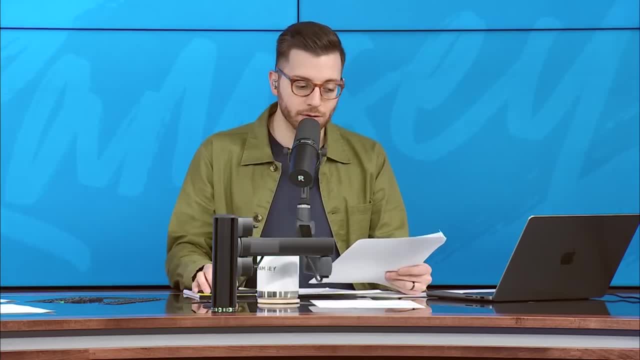 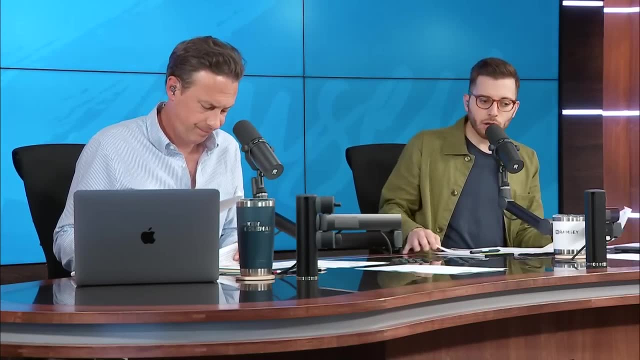 37 years And the total amount he contributes $88,800.. Now in your mind, Ken, without doing math, you're going well. Joey's got to have more money. Joey's ahead. He invested for a lot longer period of time. You would be what's known as wrong, Because 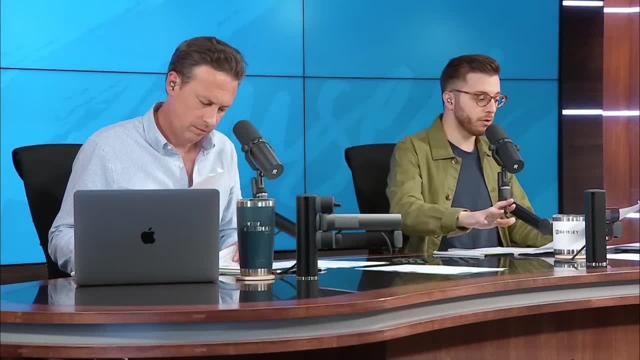 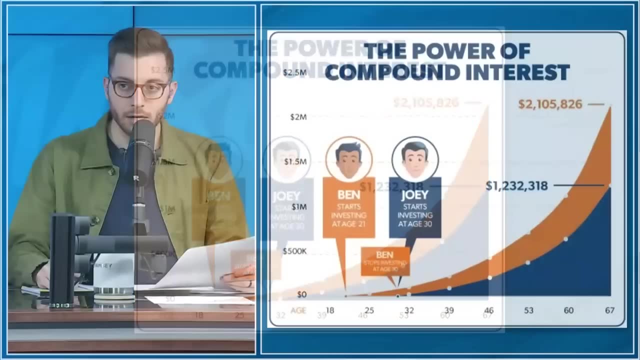 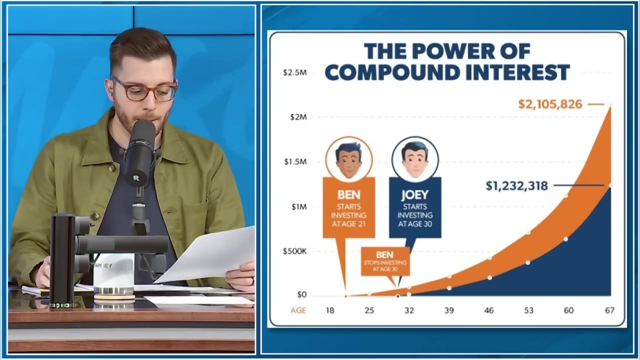 at age 67, Ben's investment- remember his $21,000 he put in- has grown to $2.1 million. Joey's investment has grown to $1.2 million. So that nine-year difference, that nine-year gap from when Ben started to when Joey started, was a difference of close to $1 million Is. 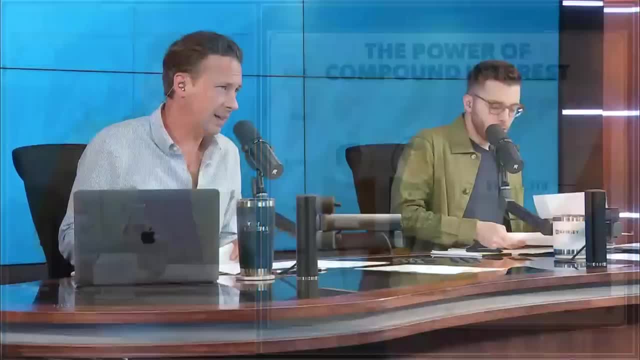 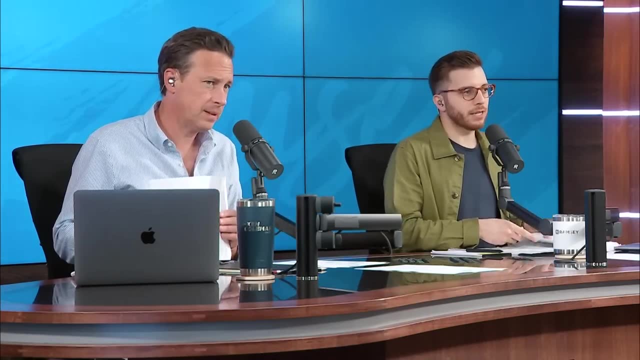 that not wild. It's crazy. Now some people hear that and they go: well, wait a second. Is it too late for me? No, Because what about the guy who started at 30?? The best time to plant a tree was 20 years ago. The next best time is today, And so regardless. 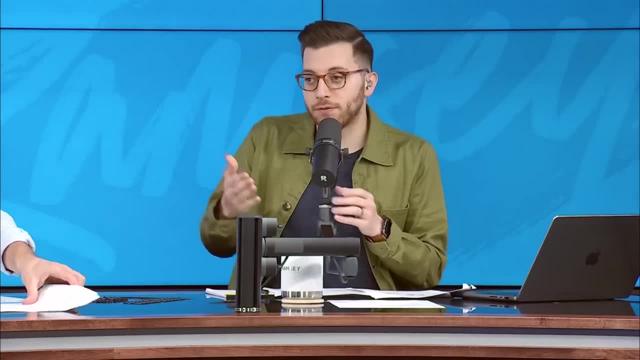 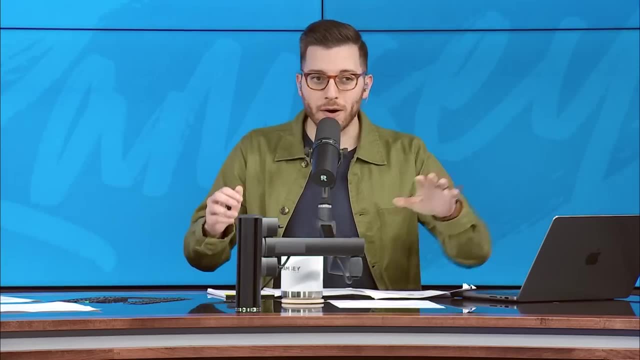 of where you're at, you got to start. And if you're 50,, well, still, if you, Let's say, it's 70 years old, You still have 20 years of compound growth to take advantage of. And if you're young and you follow this plan, you go: hey, what if I could graduate? 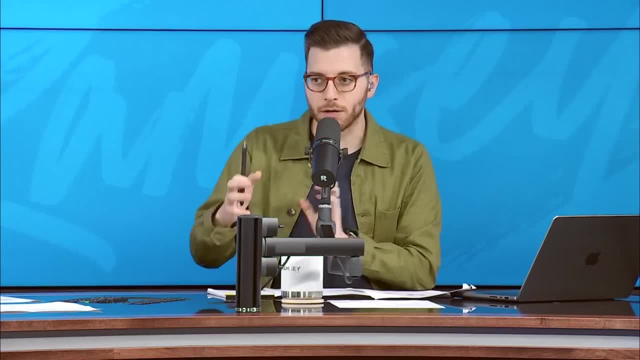 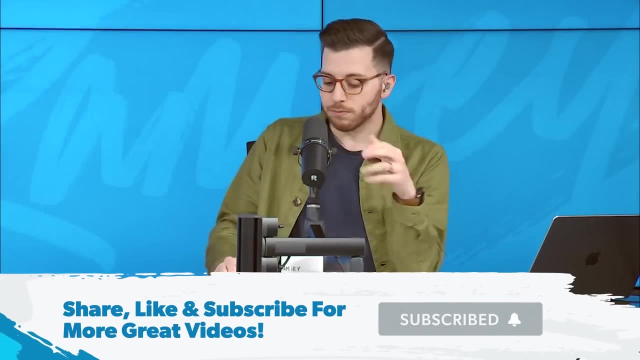 debt-free. What if I could get out of all my debt? cut up the cards, have an emergency fund, begin investing 15% With a normal income. you're going to be a multimillionaire if you just start when you're out of college, And so, regardless of your age, the key here is: